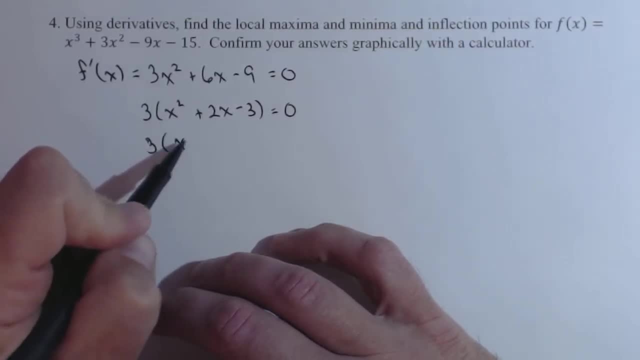 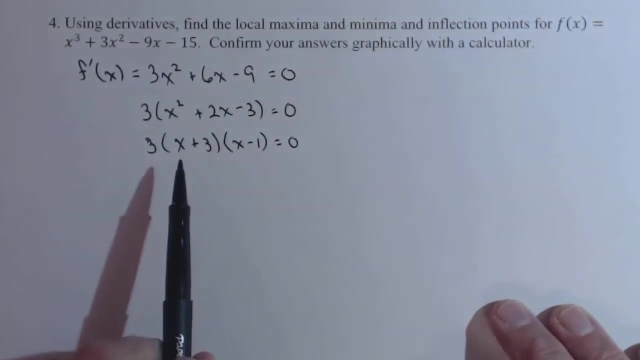 And this will factor as well into x plus 3 times x minus 1.. So right off the bat we can see that we've got two critical points At negative 3 and 1. And we can test these using the first or the second derivative test. 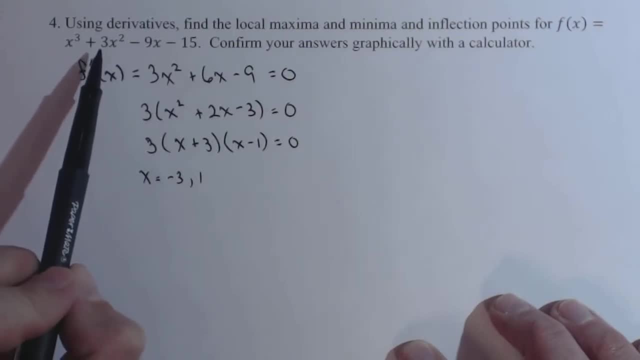 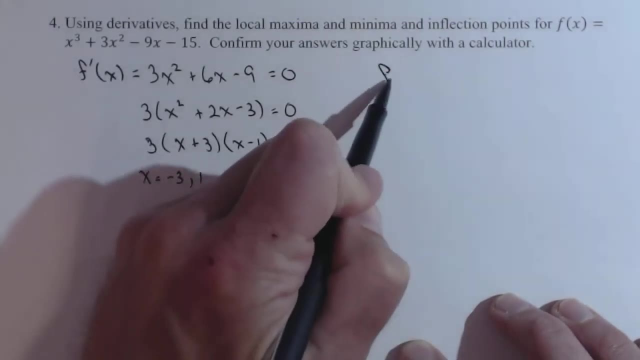 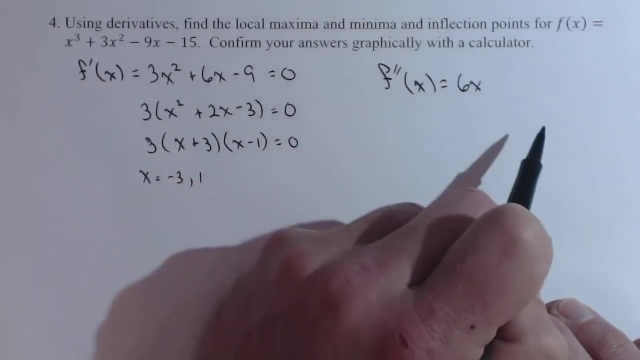 Because we're looking for maxes and mins. Since we need the second derivative anyways, let's go ahead and just use the second derivative test. So the first thing we need is the second derivative, Which again, is just piece by piece. It's going to be 6x plus 6.. 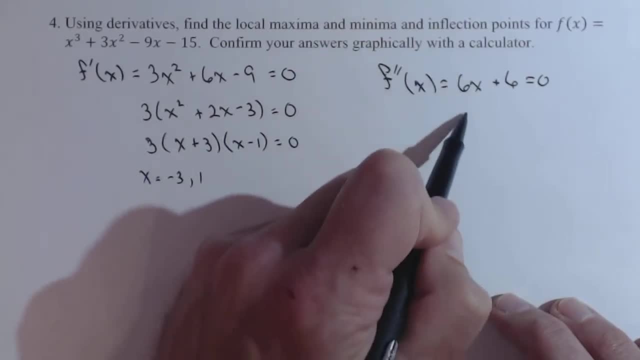 And we'll take that And we'll set that to 0 because we don't want to find any inflection points. So we have 6 times x plus 1 equals 0. So x equals negative. 1 is going to be where we might have an inflection point. 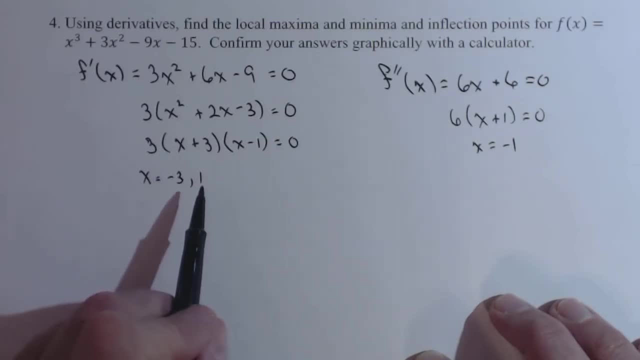 Alright, now first let's go ahead and check these and see if we have maxes or mins. And the way we do that is: we evaluate each one at the second derivative to see if it's positive or negative. F, double prime of negative 3.. 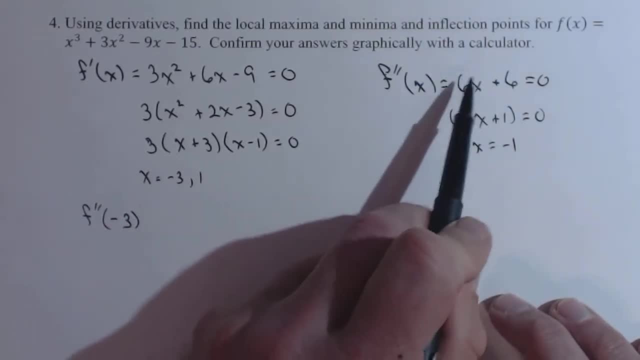 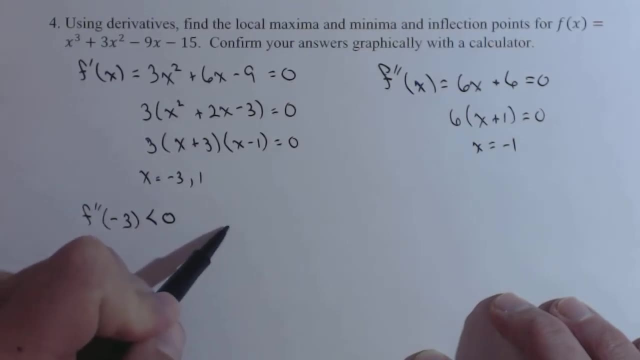 If I were to put a negative 3 in here, I get negative 18 plus 6, which is a negative number. So remember: if the second derivative is negative, just as a reminder, that means it's concave down, Which means I have a max. 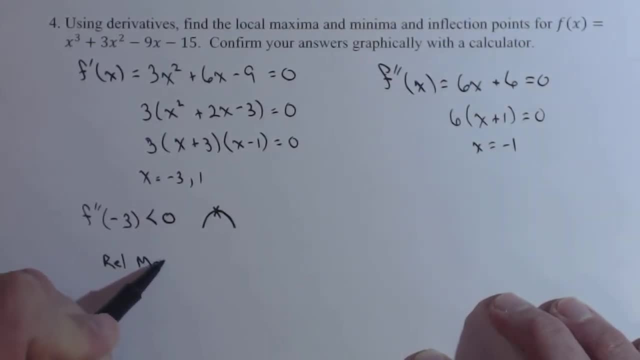 So I have a relative max at x equals negative 3. And we'll find that as a point in just a second F double prime of 1, just to verify Notice- we'll have 6 plus 6, which is 12.. So let's just use this. 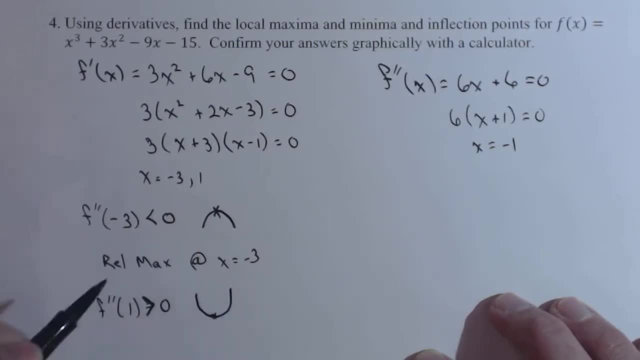 It's greater than 0. It means it would be concave up. It means we have a min. So we have a relative min at x equals 1.. Now, because they asked for a relative- these local maxes and local mins- which is also a relative max or a relative min? 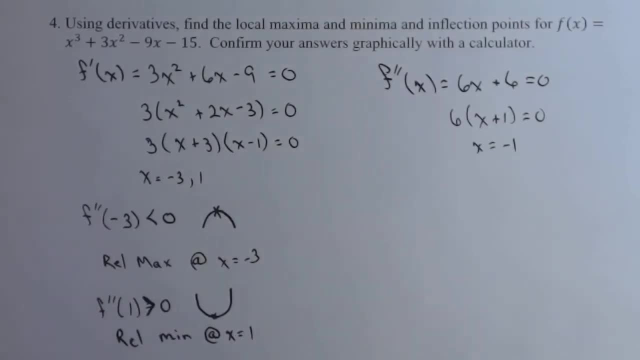 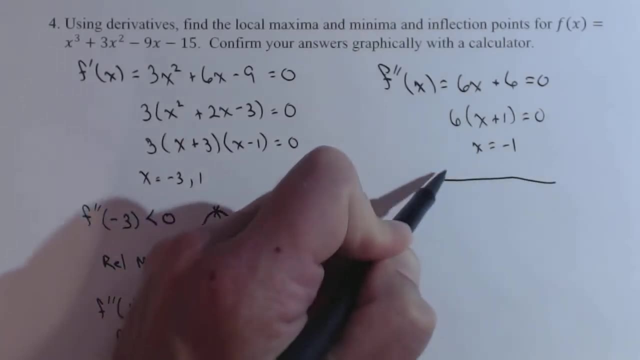 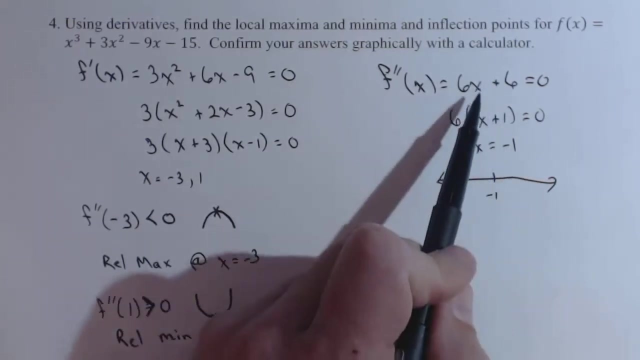 I sometimes use those terms interchangeably. We will give them as points in our inflection point. if we have one, Is it negative 1?? Well, if we were to make a number line and put negative 1 on it and check our derivative notice, if we were to put in 0, we get a positive. 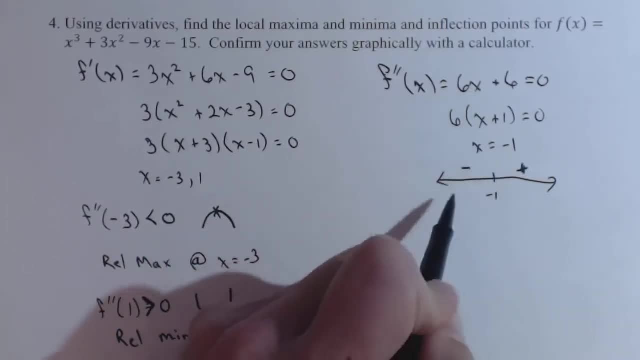 If we were to put in, say, negative 2, we'd get a negative. So our original function- this is F double prime we're testing up here. Our original function would be concave down, Concave up. So we have an inflection point at x equals negative 1.. 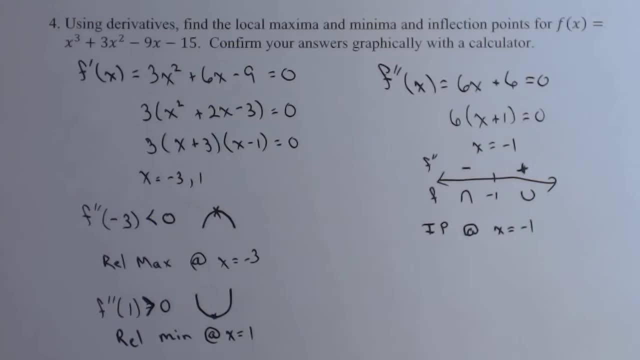 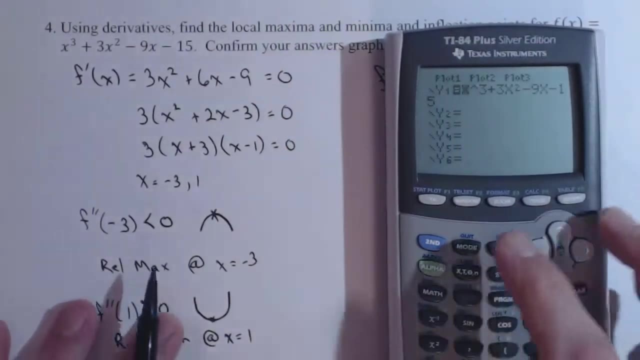 Now we need to find these as points, And so what I'm going to do is I'm going to use the calculator to help us out here, And so I've got my function in here And I have my table. I'm going to change the independent to ask. 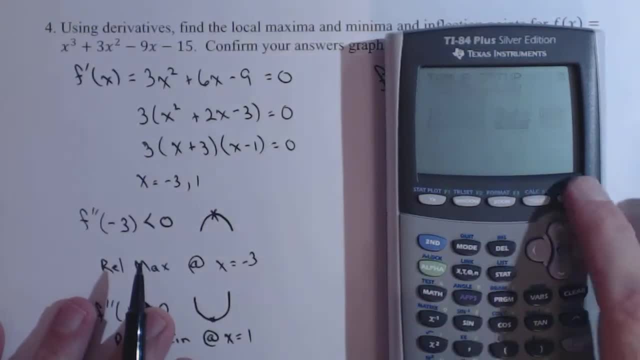 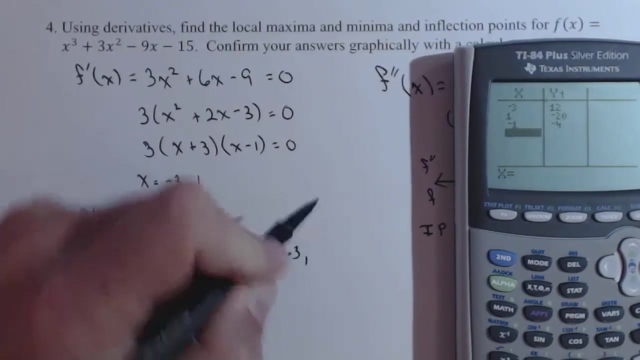 This is something that you can do to find a few values quickly And when I go to my table. I needed a value for negative 3. And 1. And negative 1.. And there are my values. So my relative max is the point negative 3 comma 12.. 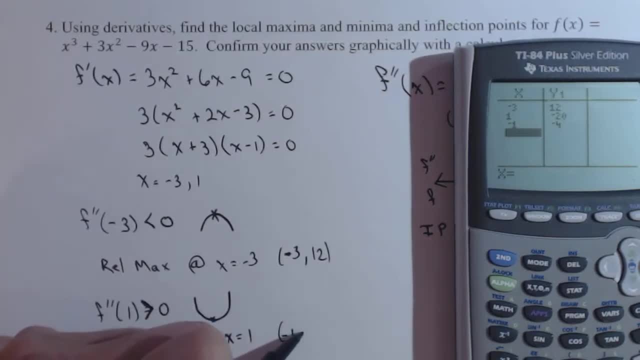 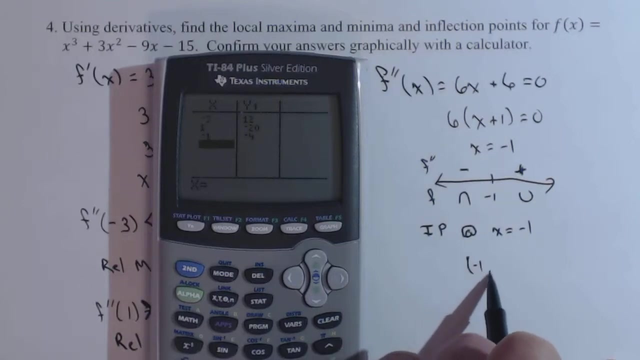 My relative min is the point negative, excuse me, not negative 1. That was for our inflection point 1 comma negative 20.. Our inflection point is at the point Negative 1 comma negative 4.. Now that we have this graph. 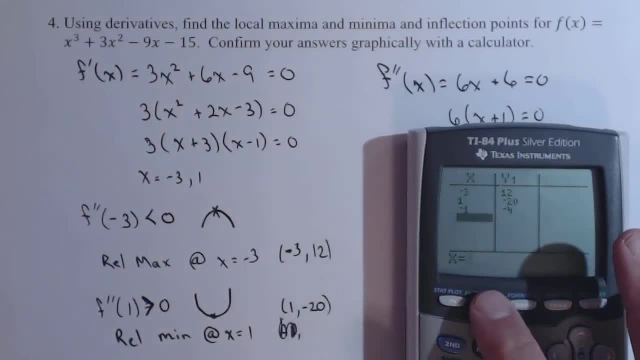 Let's confirm this graphically. We can see that to see this thing, We're going to need the window to go down to at least negative 20. And up to at least 12.. So let's give ourselves some room. And I accidentally changed the wrong setting. 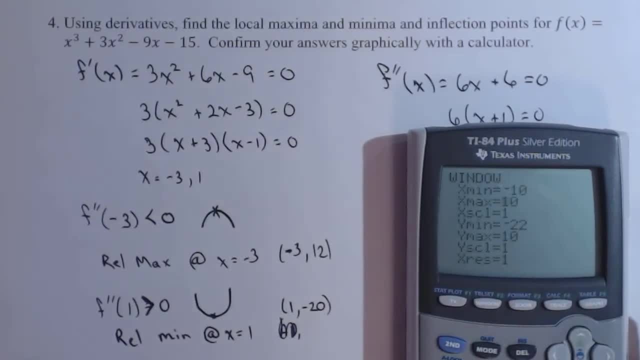 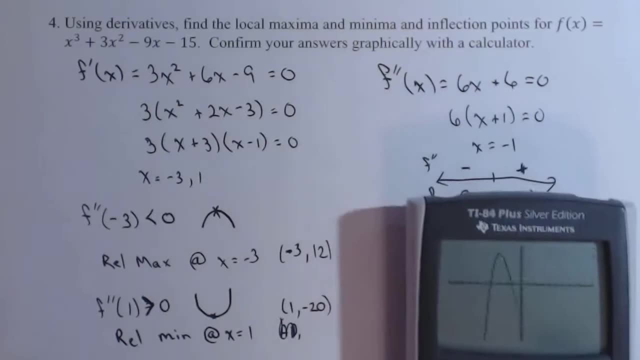 I meant to do the y max. Let's keep that at negative 10.. We wanted the y max at 15.. So you see there, We got a relative max at negative 3. It goes up to 12.. Our inflection point. 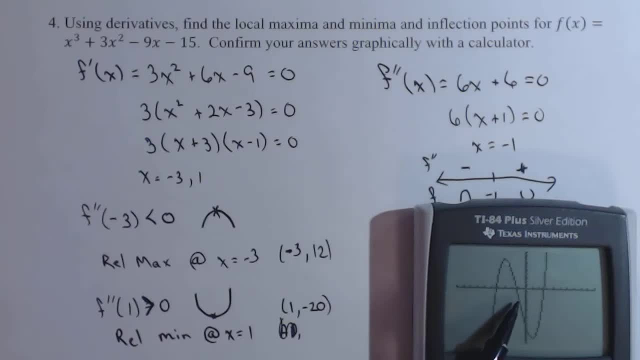 It's hard to sometimes pinpoint on a graph, But it looks like it's about at negative 1. And with a y value negative 4.. And there's our relative min sitting here at 1 negative 20..